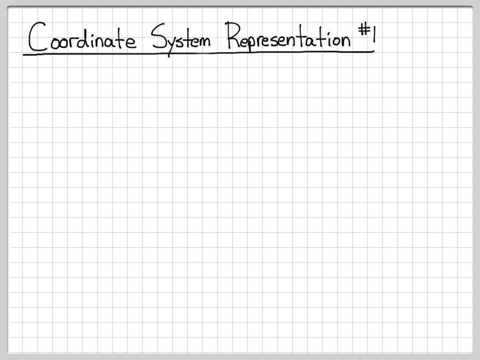 we have 1 in the direction of 1, 0, 0.. The 2 in the second coordinate tells me we move 2 units along the 0, 1, 0 direction, And then 3 in the third element would tell us that 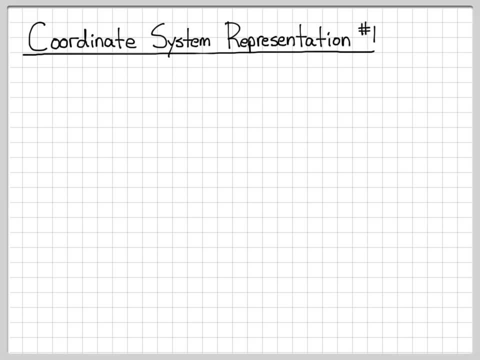 we move 3 units along the 0, 0, 1 direction, So the standard basis that we tend to work with implicitly just has a 1 in each corresponding coordinate of the vector. Sometimes we want to work in different coordinate systems though, So, for example, in this example we're going: 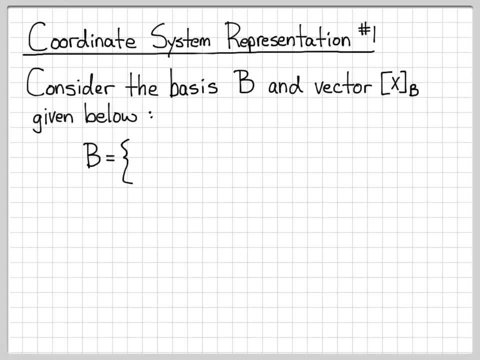 to work with a basis b That looks like this. It looks like the following: These are going to be length 3 vectors. The standard basis would be 1, 0, 0, 0, 1, 0, 0, 0, 1.. In this problem, we're going to work with a basis. 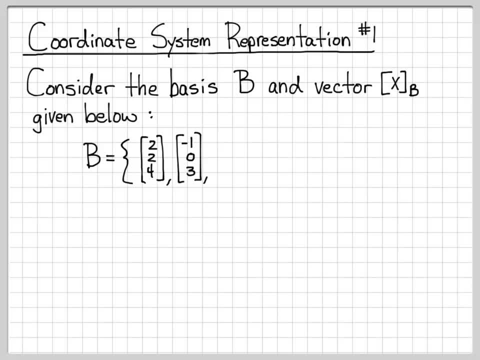 represented by 2,, 2,, 4,, a negative 1, 0, 3, and 1, 1, 1.. It turns out that these vectors are all. they are linearly independent, So they form a basis. 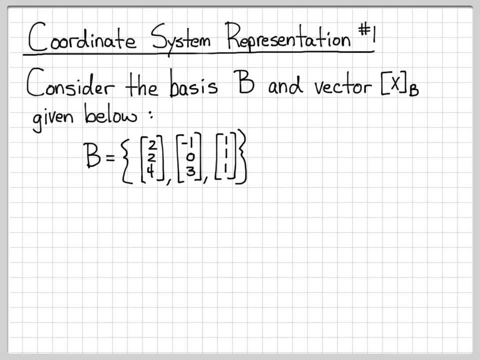 for r3. So any vector in r3 I can write as a linear combination of these vectors- And that's disappeared because I haven't fished through that quite yet- But obviously any vector in r3 that I would write as a linear combination of these vectors, those coordinates. 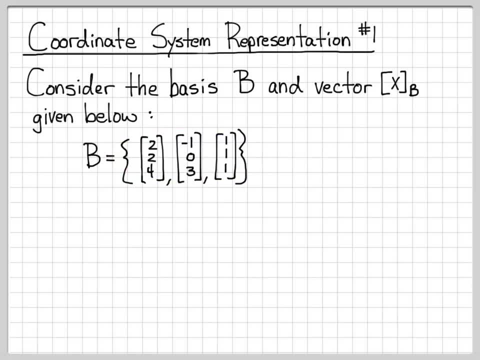 would be different than how I would write the linear combination for the standard basis, which would be the vector 1, 0, 0, 0, 1, 0, 0, 1.. So it's just a change of coordinate. 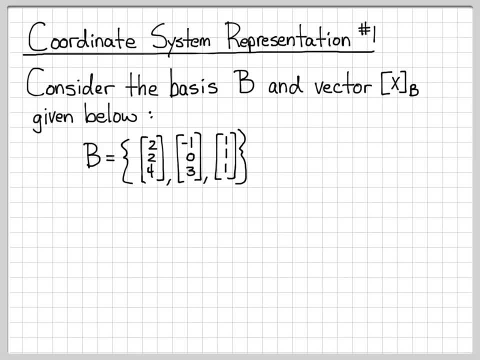 systems, so to speak, And in this first example we're going to get practice writing a vector that has been provided in this coordinate system, Because the vector is going to be more functional in this seventy-eighth this coordinate system, And we're going to translate that back into what I would call 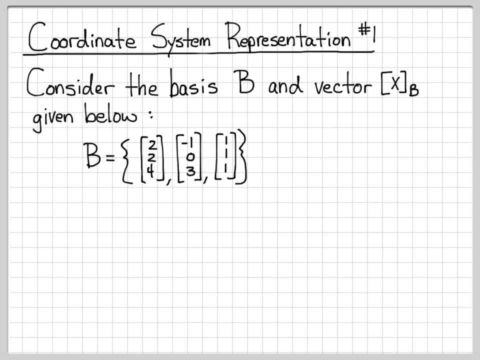 the standard coordinate system. So this is the basis that we're working with in this problem And we're provided a vector And the notation we use is x sub b And this tells us that the vector x has been written in the basis B. So anytime you see the square bracket. 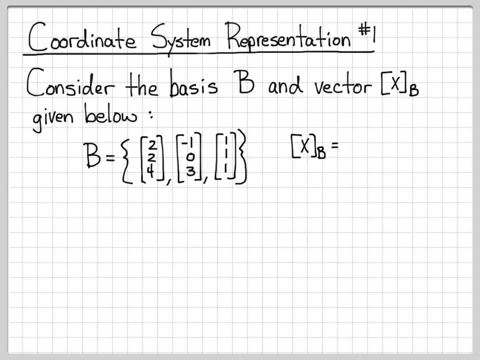 with a subscript, with a letter. that is basically just an indication that the vector has been written not in the standard basis, which is usually our implicit assumption there, But it has been written with respect to the basis B. So this vector is 2, 1, negative. 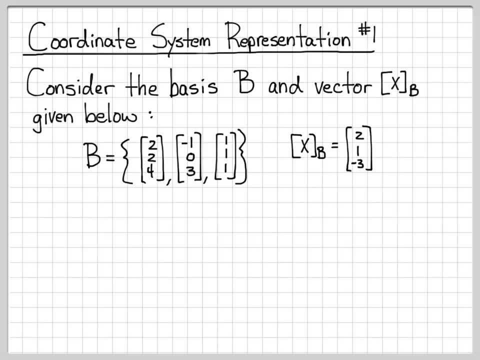 3.. So this is the representation of the vector in this basis And it really tells us to move two units along this direction and then move one unit along this direction and minus three units in this direction. So the interpretation is that the vector x has been written in the standard basis And 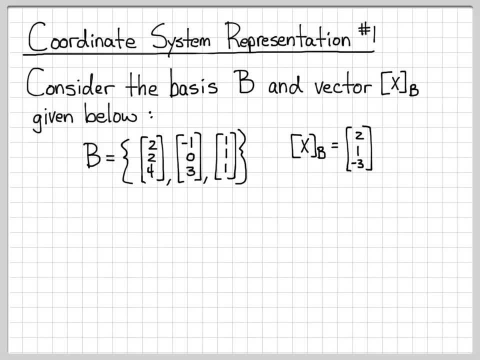 it's still very much the same. It tells us how many units we've moved in each direction, But the directions aren't the standard directions. They're these directions specified by this new basis B. OK, So that's a little explanation about some of the things we like to do in. 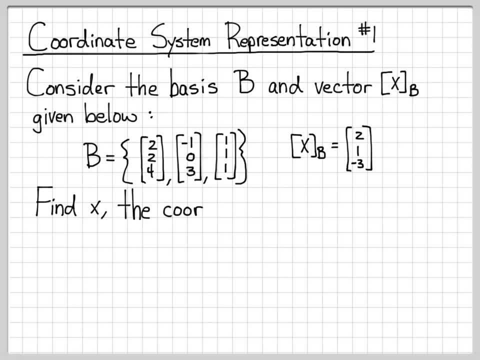 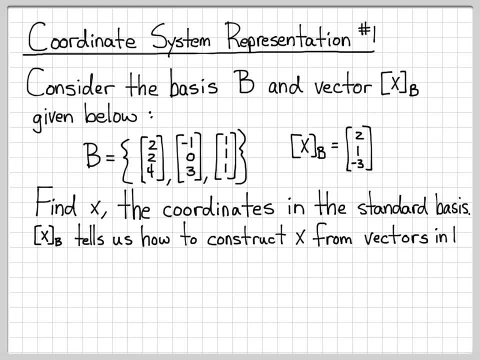 that X sub B tells us how to construct X from the vectors in B. So let's take a look at this. Let me go ahead and write down X sub B and let's think about what each of these entries means. 2 tells us to move, like I said, 2 units in the B1 direction. 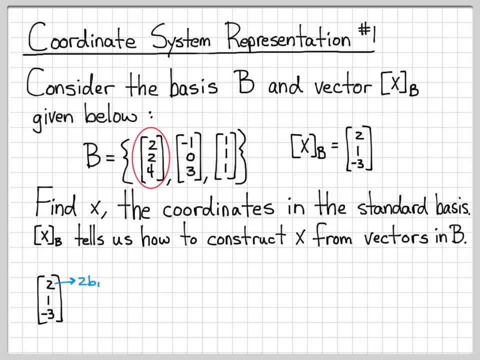 So this vector right here is a vector in the standard basis- 2,, 2,, 4, obviously, And this first coordinate tells us to move 2 units in that direction. The second coordinate tells us to move 1 unit in the B2 direction. 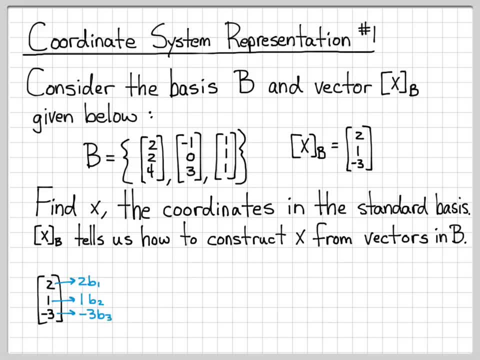 where B2 is this second column And a negative 3 tells us to move 3 units in the negative direction of B3, where B3 is this third column of the basis B. So we can go ahead and form this linear combination now to figure out what X is. 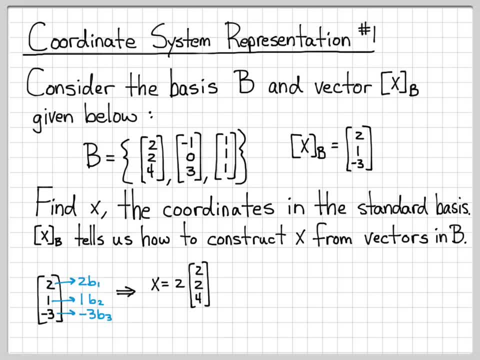 X is going to be 2 times this first column, plus 1 times the second column, plus a negative 3 times the third column. So if I go ahead and do my algebra there, 2 times 2 is 4,, 2 times 2 is 4, times 2 is 8.. 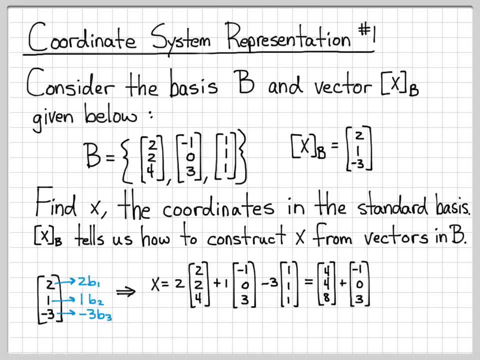 1 times the second vector. just gives me the second vector And then a negative. 3 times the third vector gives me a negative. 3 is everywhere. If I add all these coordinates up, 4 minus 1 minus 3 gives me a 0..